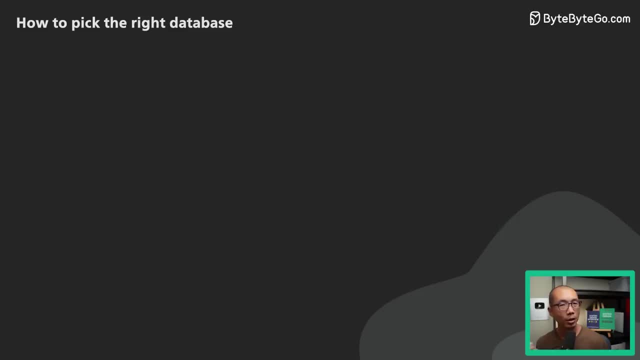 that would give us more breathing room. Can we put a cache in front of it and give us a few more months of runway? Can we add read replica to offload some read load? Can we short the database or partition the data in some way? Maybe the data is naturally siloed and sharding is an acceptable solution. The bottom line is this: Migrating a live production database is risky and costly. We better be sure that there is no way to keep using the current database. 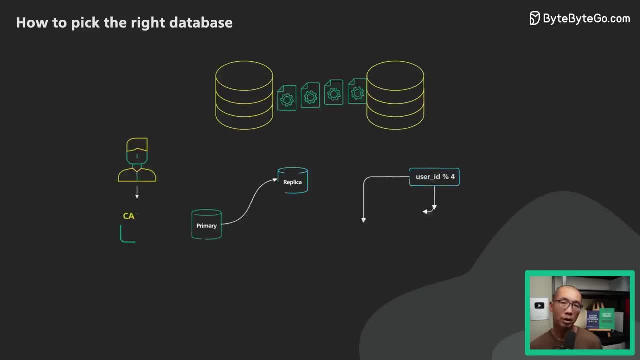 Okay, we have exhausted all avenues for the current database. How do we go about choosing the next one? We developers are naturally drawn to new and shiny like moths to a flame When it comes to databases. though boring is good, We should prefer the ones that have been around for a long time. 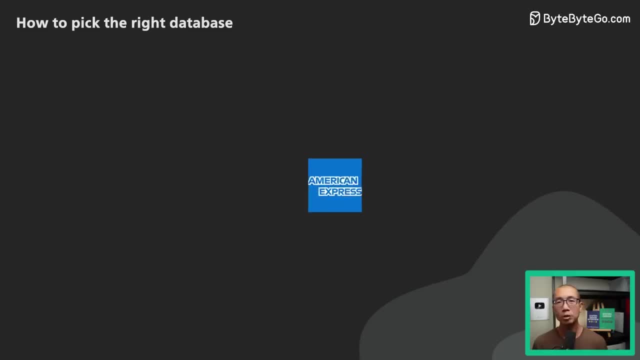 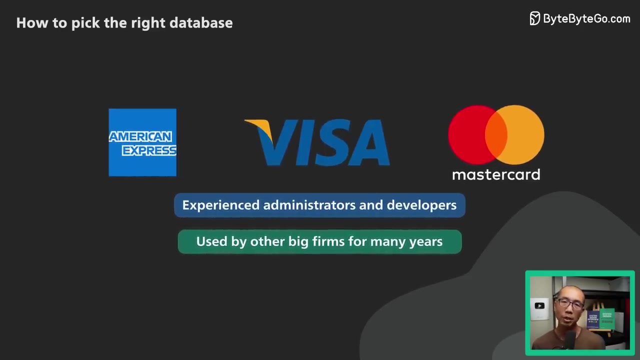 and have been better tested. Depending on the industry we are in, our posture could be a little different. Banking and finance is a lot more conservative, for example. Whatever it is, there should be a ready market of experienced administrators and developers for the database we are considering. 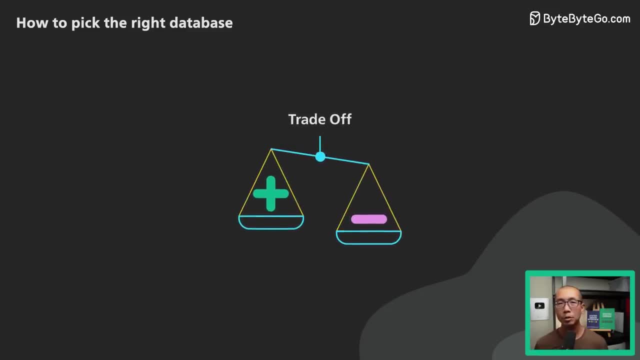 Software engineering at scale is about trade-offs. When it comes to databases, it is even more true. Keep in mind: there is no free lunch. Be weary of outrageous marketing claims. Infinite, effortless horizontal scalability comes with a hidden cost. Dig deep to find where that cost is hiding. 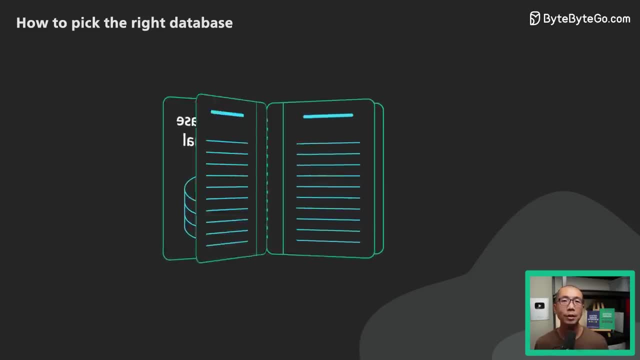 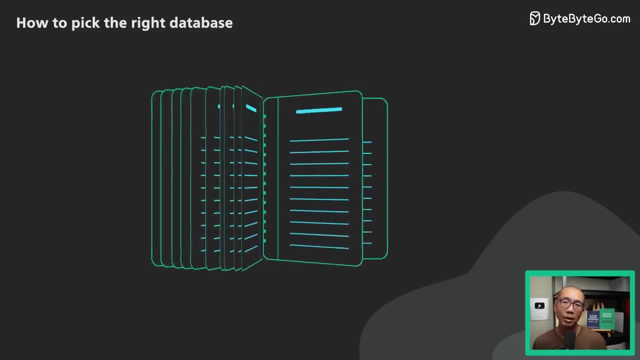 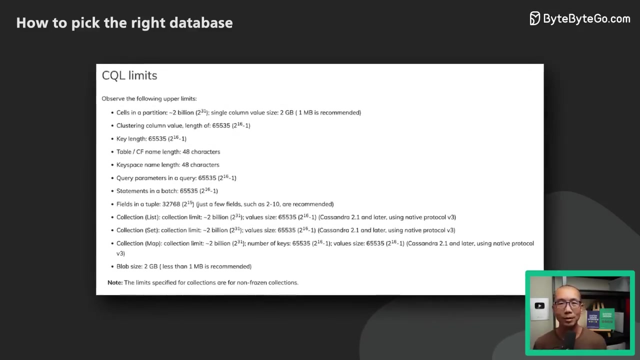 Instead of reading the shiny brochure, go read the manual. There is usually a page called Limits. That page is a jam. The FAQ section is also very useful. These pages in the manual are where we learn the real limits of a new database. 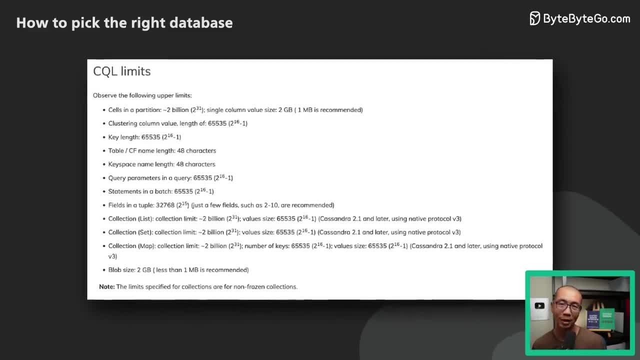 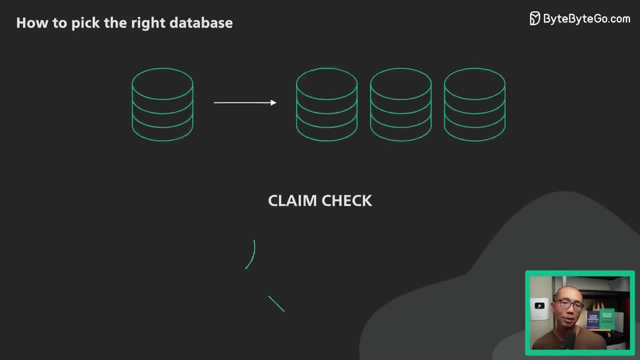 its design constraints, the fine prints, so to speak. If the brochure promised infinite horizontal scalability, these are the places to fact-check those claims and to find the catch. In our experience, the fancier the claims, the longer the disclaimers in the back. 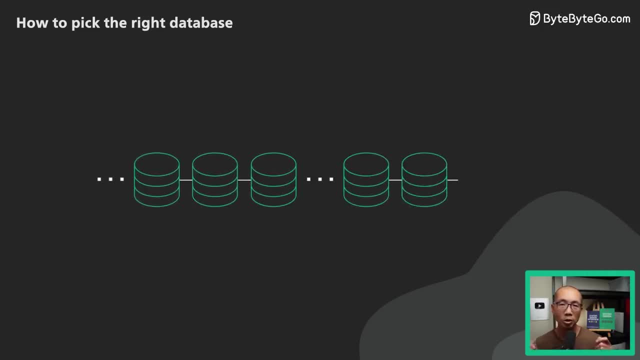 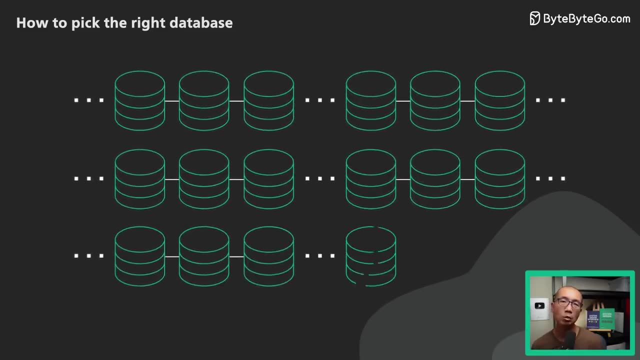 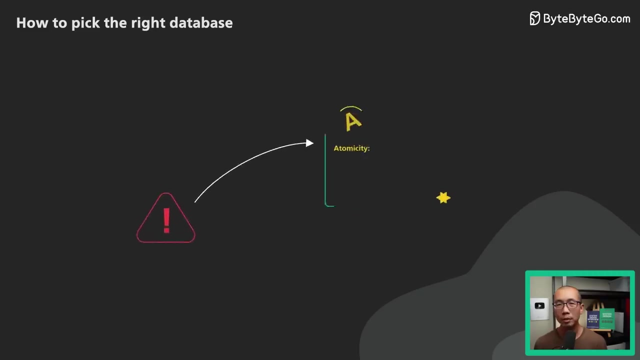 For example, many NoSQL databases support much higher scale than the trustee of NoSQL. They often claim to support near-linearly horizontal scalability. Here are the common trade-offs that come with them: 1. They eliminate or limit transactional guarantees. 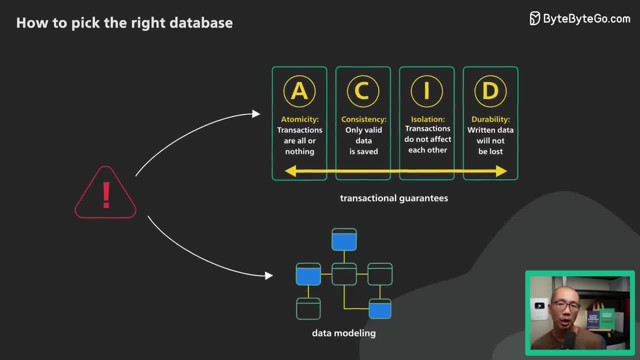 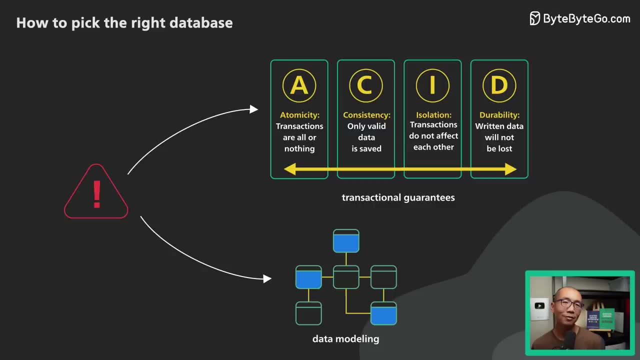 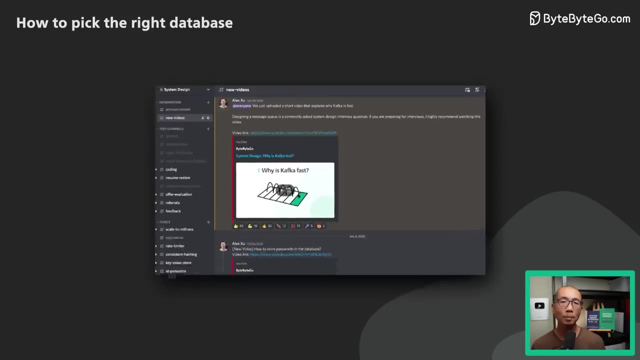 2. They severely limit data modeling flexibility. There are no queries across data entities. The data is highly denormalized, where the same piece of data is stored in many collections to support different data access points. These are the major patterns To learn even more about a particular database. 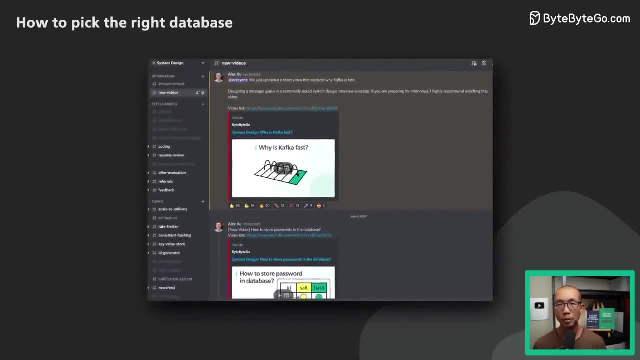 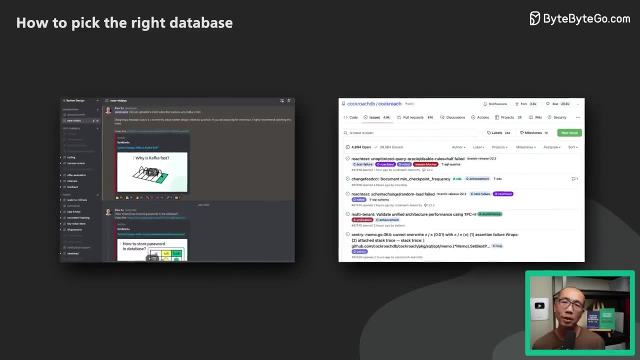 join the chatroom. ask lots of questions For open-source projects. read the GitHub issues. Learn as much as possible about the candidate now. The investment is relatively small at this juncture. Once we narrow down the database options, what's next? 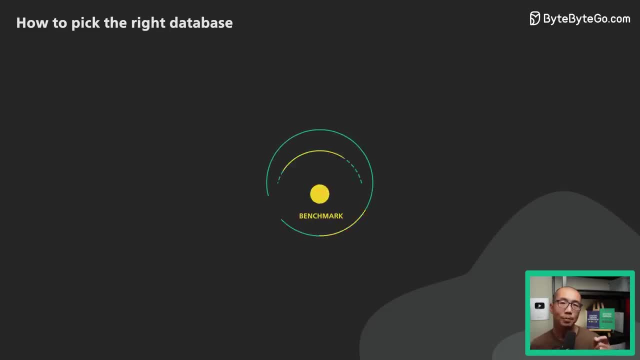 Well, let's have a shootout. Create a realistic test bench for the candidates using our own data, with our own real-world access patterns, and share them with your friends patterns. We have the data right. After all, our current database is bursting at the seams. 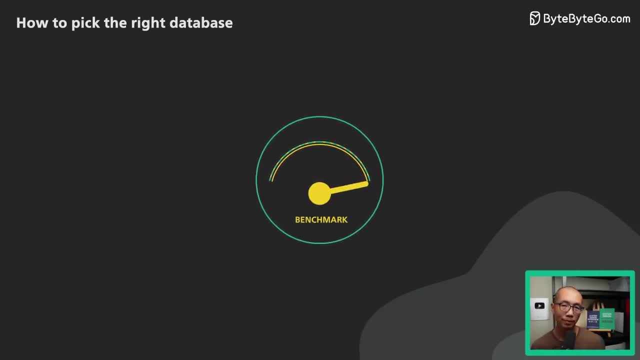 so getting some representative data should be possible. Yes, this is costly and it could take weeks, but we cannot afford to skip this step. Migrating a production database is risky and it takes a lot more work than benchmarking If we are staking our career on this new database. 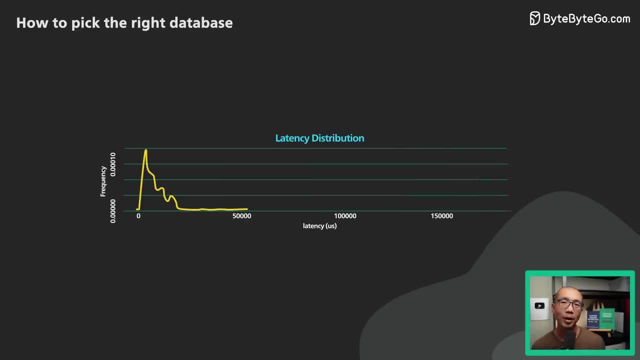 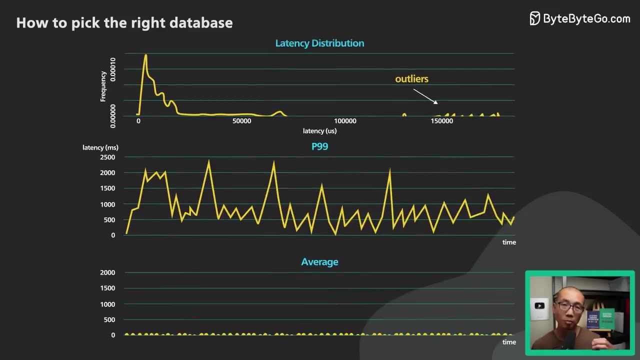 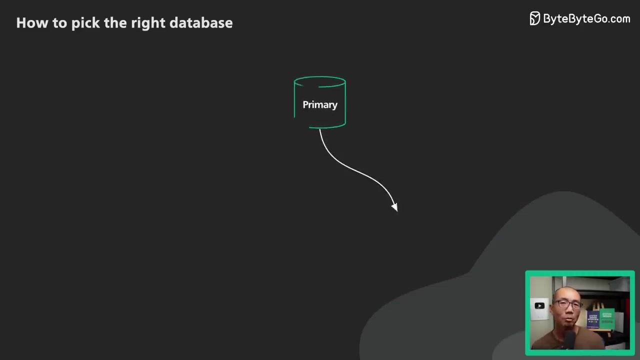 let's make sure it will work. During benchmarking, pay attention to the outliers. Measure P99 of everything. The average is not meaningful. Try hard to replicate the real workload and then push it further and see where it starts to break. Try some of the more risky operational. 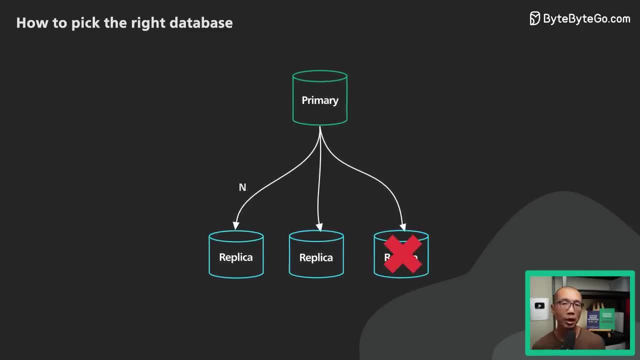 tasks like failing over a node or testing for data corruption during network partitions. Try up- or down-sharding, if it is applicable. After everything checks out, we can start to run the project. All the data is in a new plan, the migration carefully. Write out a detailed, step-by-step migration plan. 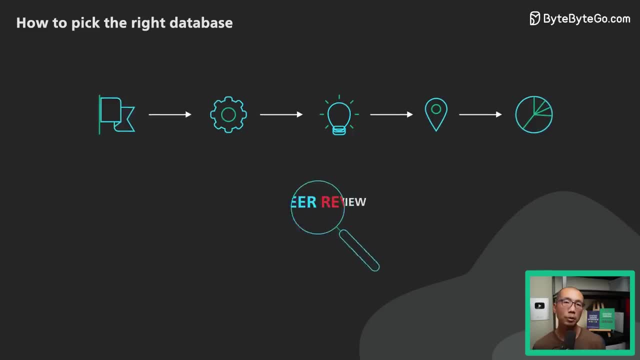 Have your peers review it thoroughly. If possible, migrate a small service first and learn as much as we can from that. Picking the right database is not glamorous and there's a lot of hard work involved. Migrating to a new database in. 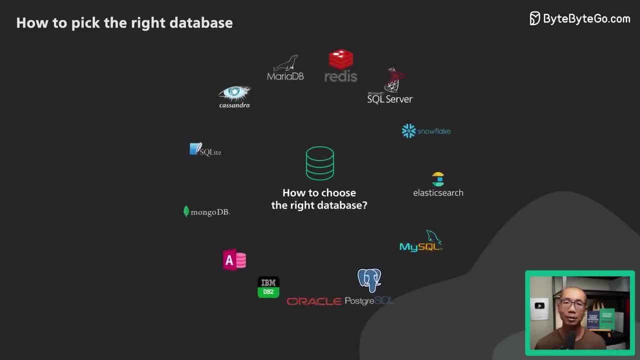 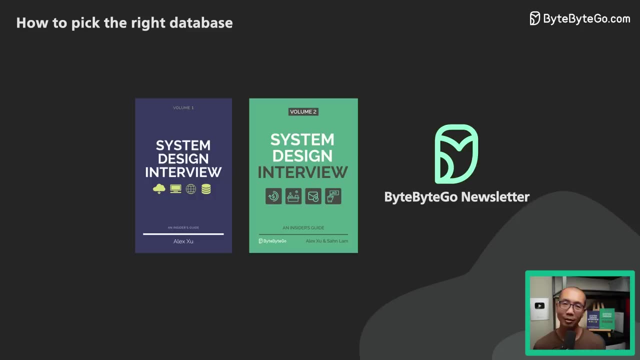 the real world could literally take years at high scale, So good luck. If you would like to learn more about system design, check out our books and weekly newsletters. Please subscribe if you learned something new. Thank you so much and we'll see you next time.